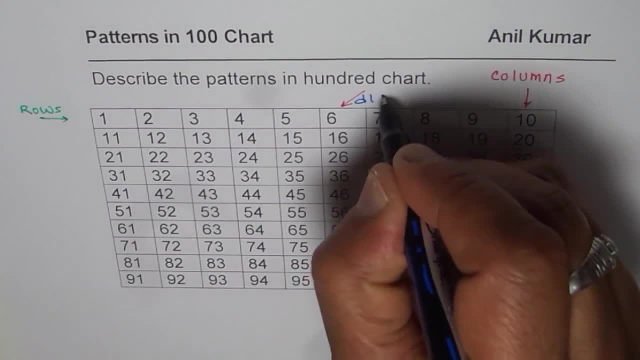 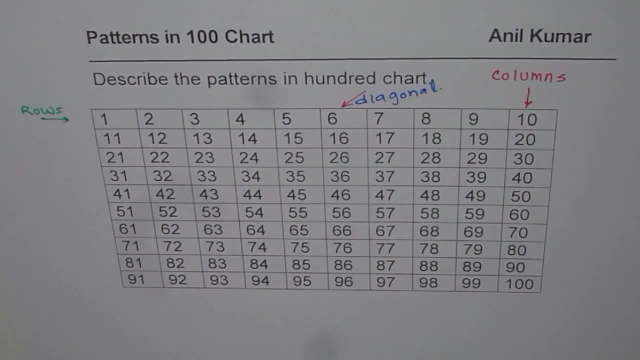 write as a diagonal, So you can use these terms to describe the patterns which you see in this chart of 100 numbers, right? So let's begin with rows. What do you notice? If you follow this row, every number is increasing by 1, right, 1, 2,, 3,, 4,, 11,, 12,, 13,, 14,, 21,, 22,, 23.. So, if you follow the rows, 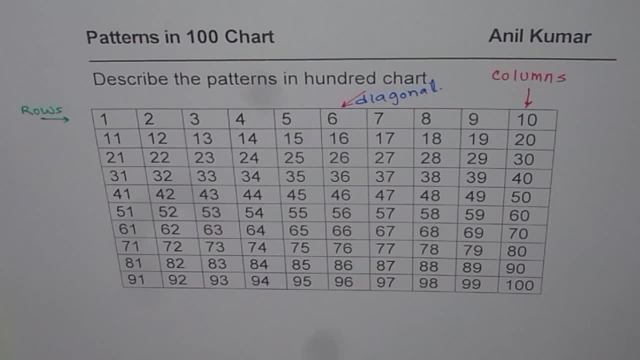 the numbers are increasing by 1.. Correct, How about columns? If you follow a column 10,, 20,, 30,, 40, the numbers are increasing by 10s. any column: 9,, 19,, 29.. 29 plus 10 is 39.. 39 plus 10 is 49. And then as you continue. 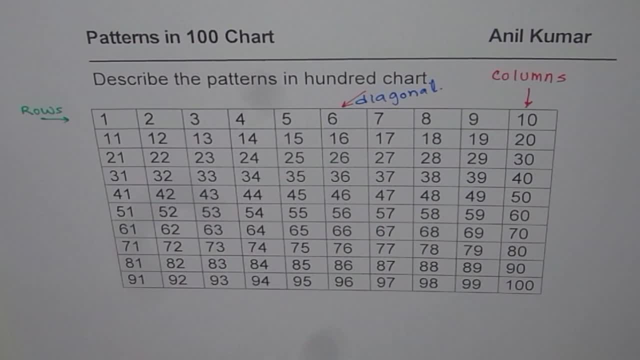 adding 10s, you get more numbers in the same column, right? So the pattern in a column is that the numbers increase by 1.. 10, right? One more thing which you notice in a column is that these are the 1s place. 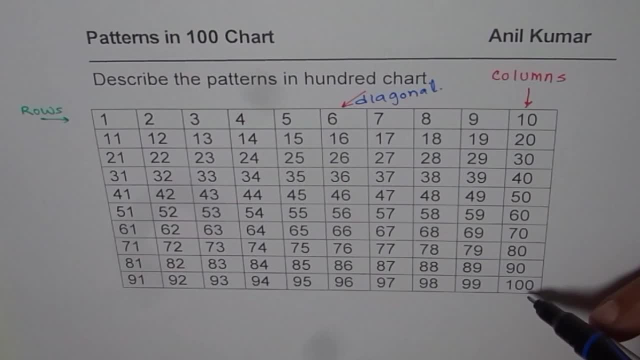 0, 0, 0,, 0,, 0, 0.. They remain same right, But 10s place increase by 1.. 1,, 2,, 3,, 4,, 5,, 6,, 7,, 8,, 9,, 10.. Do you see that? Okay, 10s place here could be treated as 0, then 0,. 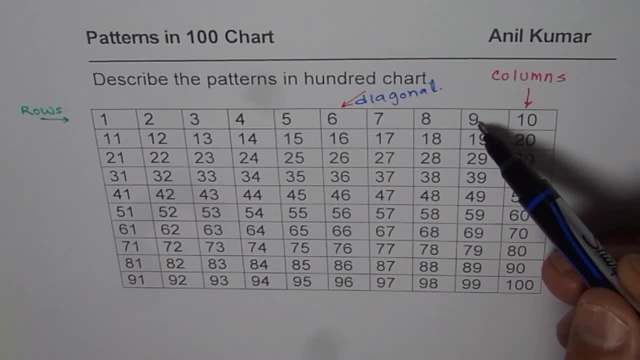 1,, 2,, 3,, 4, and so on, But the 1s place is 9s. So in these columns 1s place remains the same And 10s place increase by 1 each time as you go down. correct, That is what. 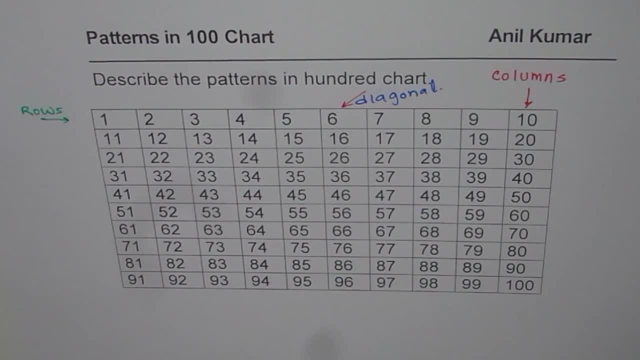 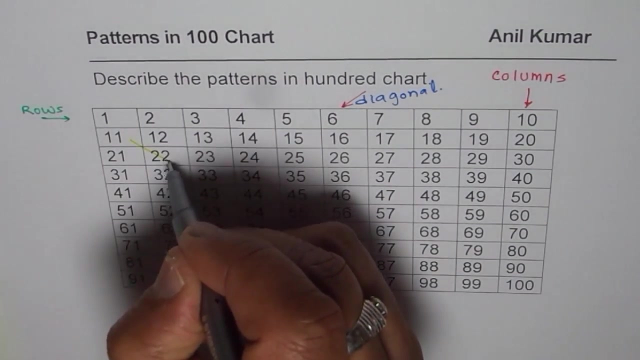 is meant by saying added 10, right? So when you add 10, 10s place increase by 1.. Now can you explore some patterns diagonally. One diagonal is very important. Look at this tag. What do you notice? 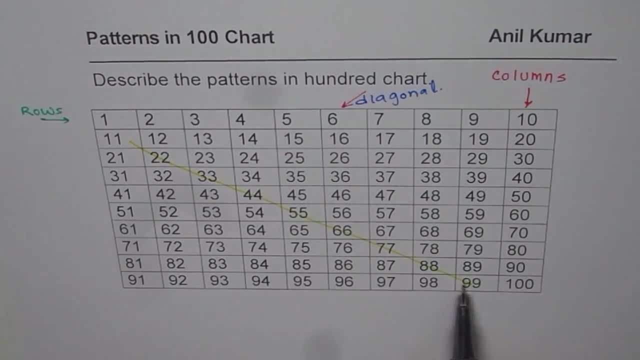 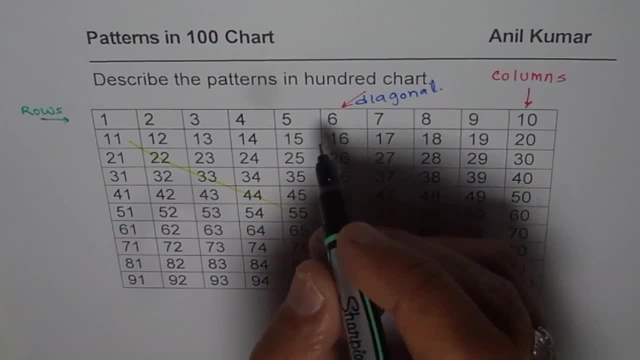 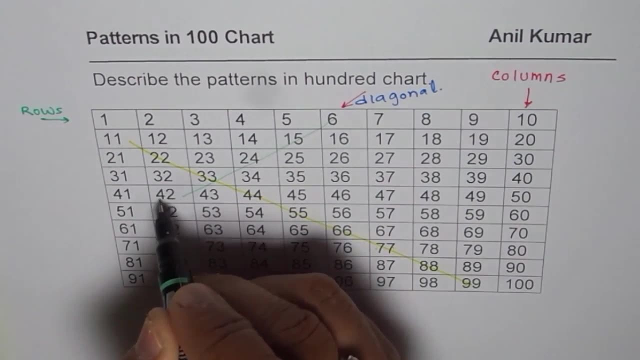 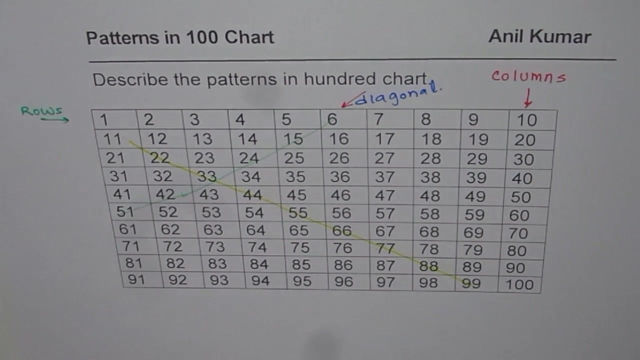 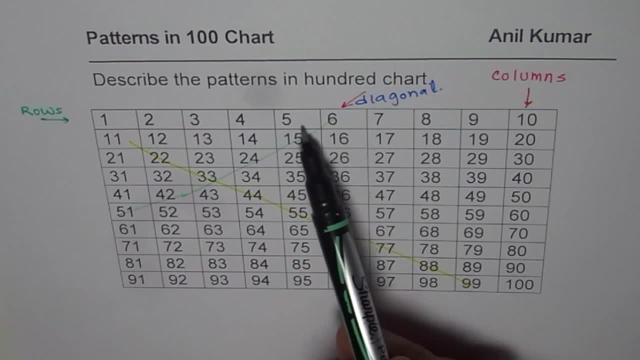 So if you move diagonally towards left side and down, the sum of digits is same: 6.. 1 plus 5 is 6.. 2 plus 4 is 6.. 3 plus 3 is 6.. 4 plus 2 is 6.. 5 plus 1 is also 6, right. 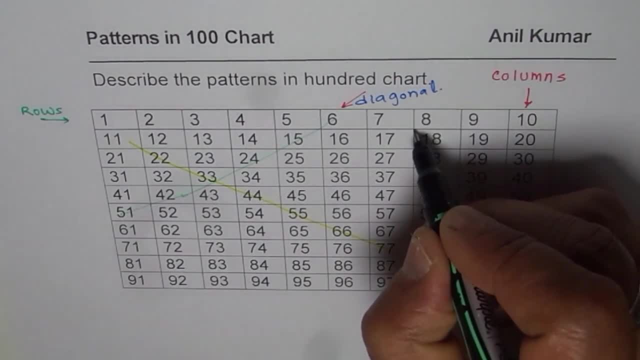 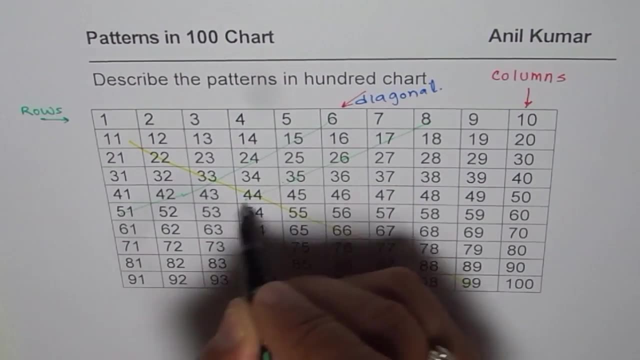 You can try it out with any other diagonal starting with 8, right, For example 8, 17.. 6 plus 2 is 8, right. 3 plus 5 is 8.. 4 and 4 is 8.. 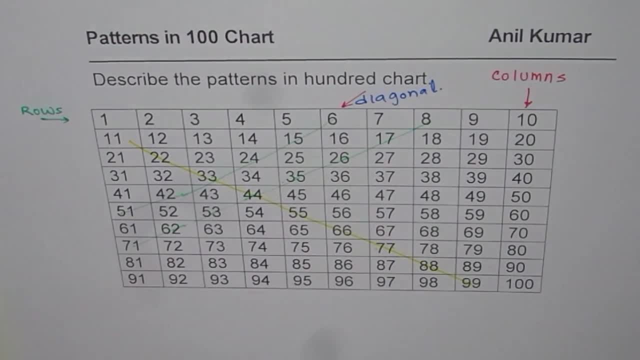 5 and 3 is 8.. 6 and 2 is 8.. 7 plus 1 is also 8.. So when you move left and down, the pattern is that the sum of digits is same. right, So you can pause the video copy. this Sum of digits remains same if you move left and down along a diagonal, correct? 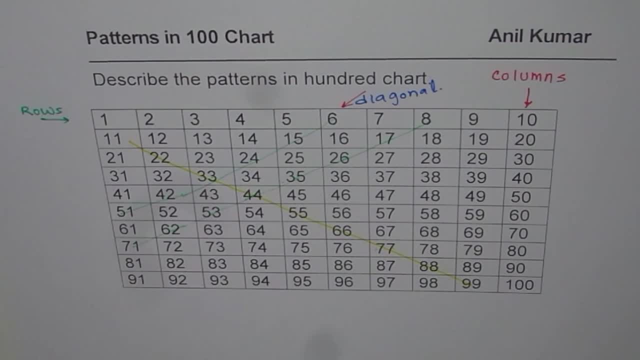 Okay, now let us see what happens when you move towards the right side from any position. Let us say, if you move right and down, so from 41 to 52, then 63,, 74,, 85 and 96.. What is happening in this diagonal? 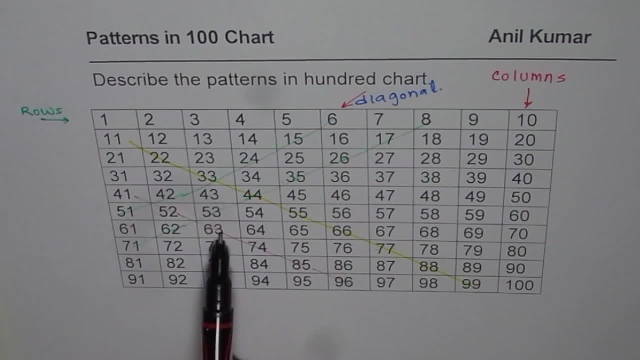